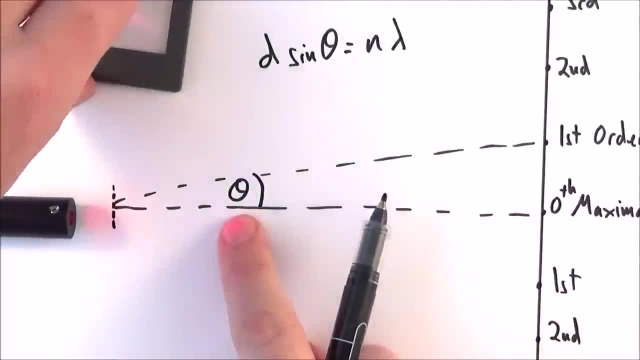 very well in the lab. Now, the good thing about using a diffraction grating to measure the wavelength of light over the two-slit is that we can measure the wavelength of light over the two-slit experiment. is that there's so many different gratings here. it lets a 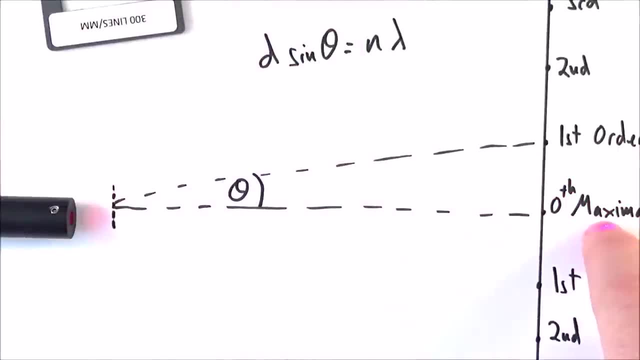 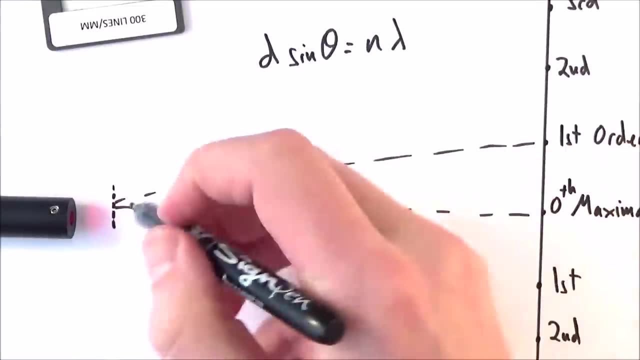 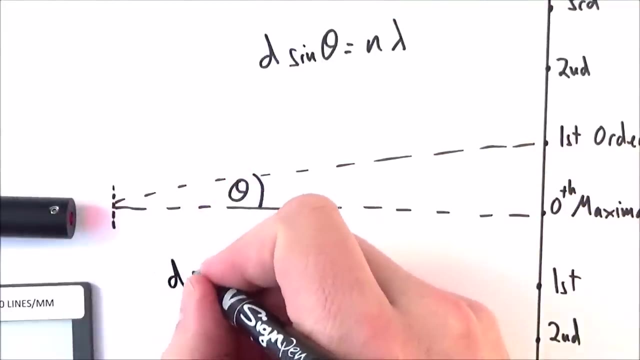 lot of light through, So that means it's very easy to see the bright fringes that we see over here. We can also look at the separation of the fringes. Now on the slide here there are 300 lines per millimeter, So d is equal to the distance between the slits. Now if 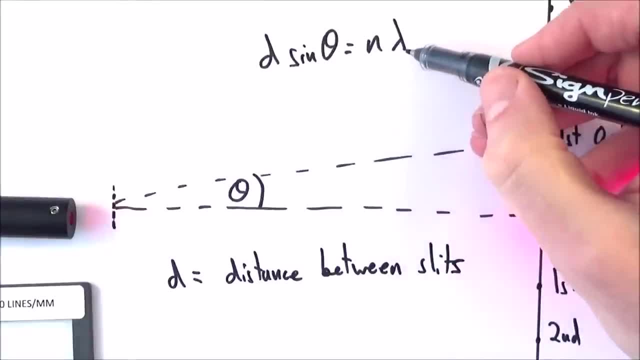 we look at the distribution, we can see that the right-hand side, which is the right-hand side of the graph, is the right-hand side of the graph And on the right-hand side we can see the right-hand side. So on the left-hand side we can see the right-hand side. 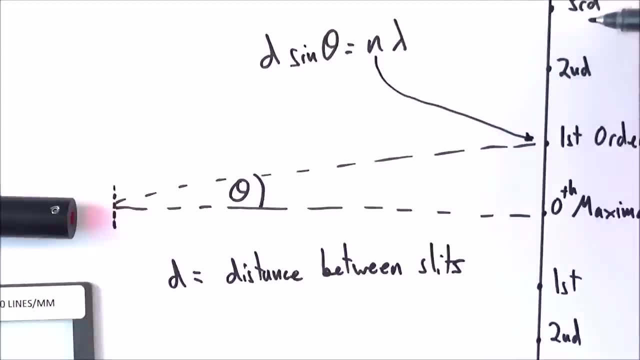 So we can see that we have an angle. theta- Okay, The lambda over here- is the wavelength of the light. Theta is this angle here And n refers to the order of the maximum. So we might have n equals 1,, n equals 2, or n equals 3, and so on. Now, if we set this up in the 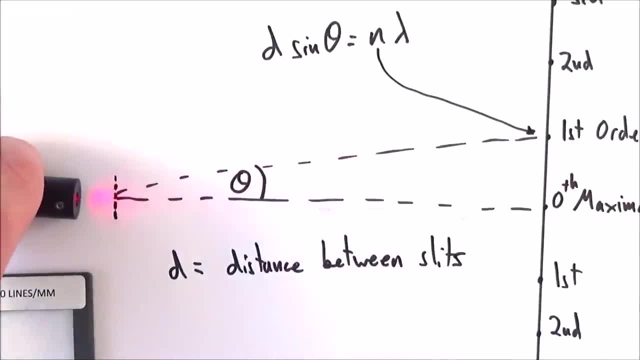 lab, we may want to find out or just confirm the wavelength of light. If you set this up, so you've got a large enough distance to measure the angle. theta. it's fairly straightforward, because we've got a triangle here with a right angle, We can measure this distance and we 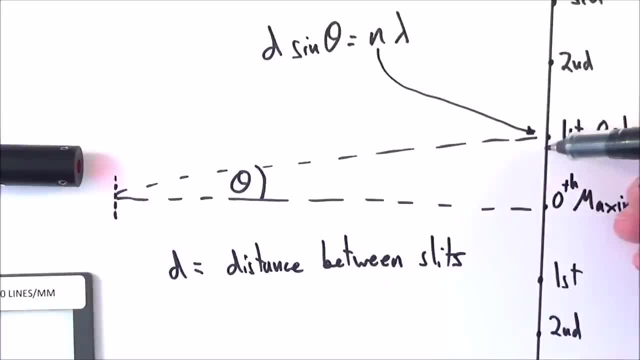 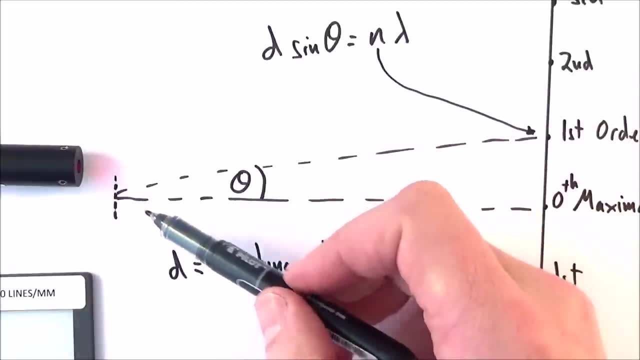 measure that distance and therefore we can calculate theta. We can maybe look at the distance from maybe the 0th to the first or second order maxima, and then we can very easily work out the distance between the slits. If we know all of that, we can work out the wavelength. 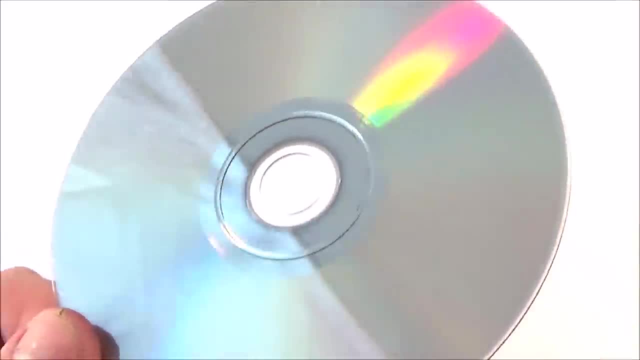 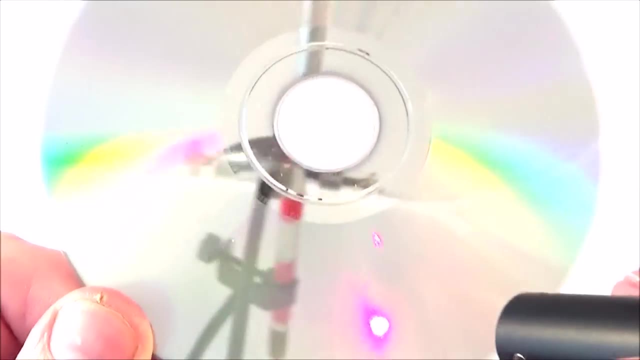 of the light. So why is it that this frozen DVD, as horrible as it is? why does that leave a beautiful rainbow of light, But yet if I shine red light on it from the laser, there's no other colours showing. Well, the reason for that is this acts as a reflective diffraction. grating. 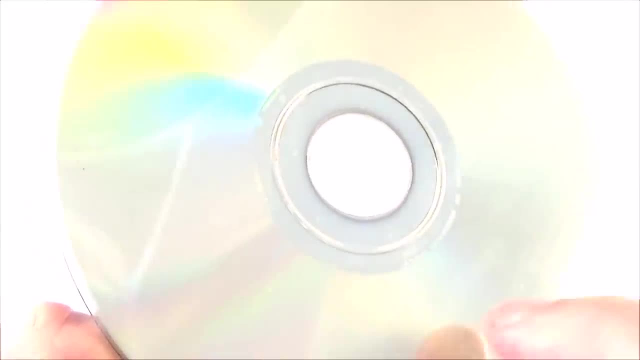 What there are are thousands and thousands of very, very small lines, so many hundreds of lines per millimetre, and that acts in the same way as the diffraction grating that we saw, where we just had the light going straight through, And it's the light that's reflected. 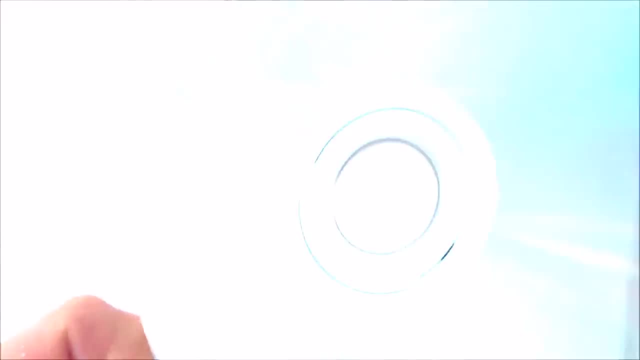 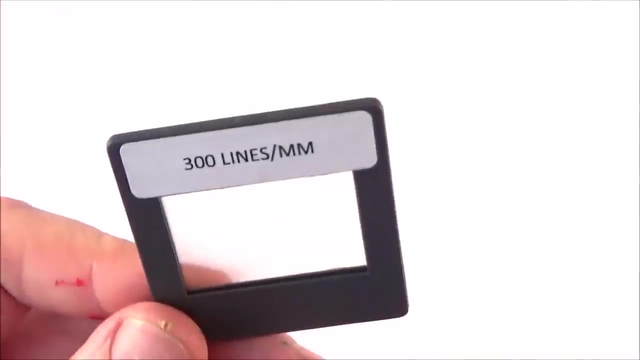 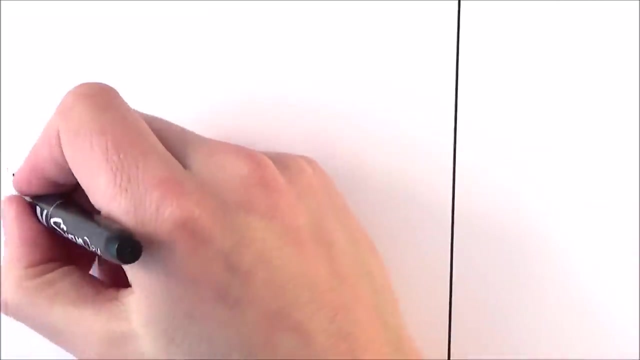 comes out in the different colours. So if we can think about having a rainbow from white light on this, what would happen if we shone white light through our diffraction grating? What we tend to find is there's a bit of a sort of rainbow towards the edge When you shine white light through.